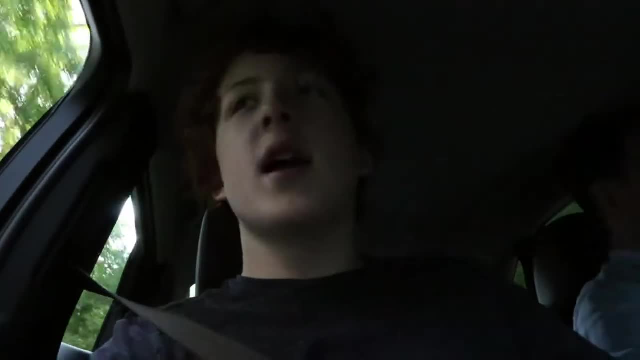 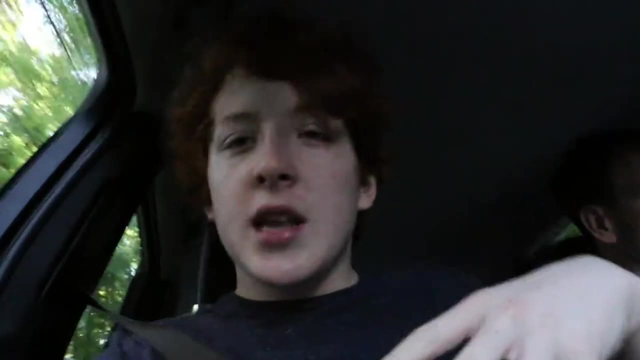 help do research about if we're going to a point, what kind of, what sort of jurisdiction that area is under. that would be really great because you can go to the Wikipedia page and try to find some line somewhere in the page about what park or what kind of area that 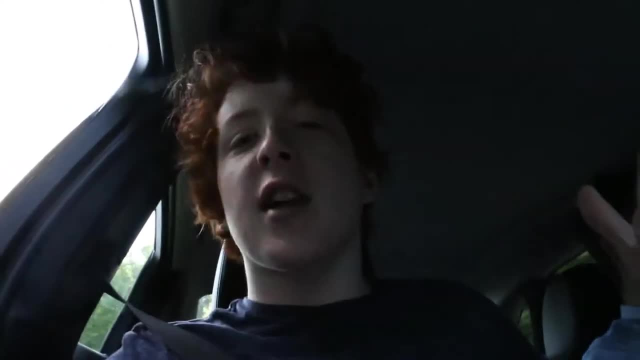 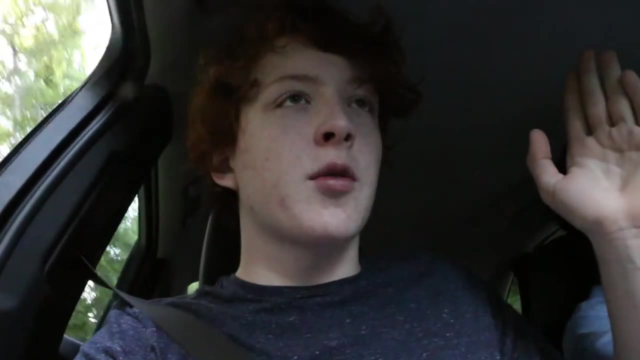 or forest it's in, but there's really no easy way to find out that I've been able to find. It really requires a lot of deep digging and I really wish you could just pick a point. Anyways, if that exists, someone should tell me. Otherwise I don't know, Just guesswork. 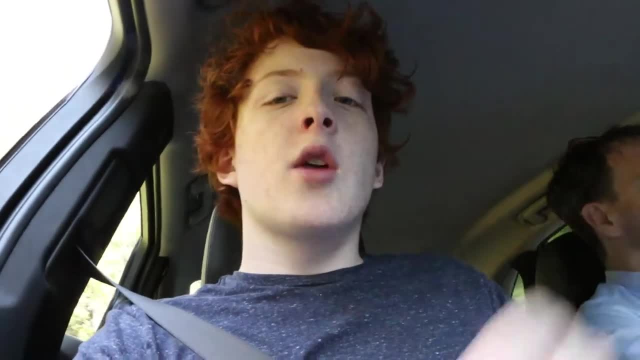 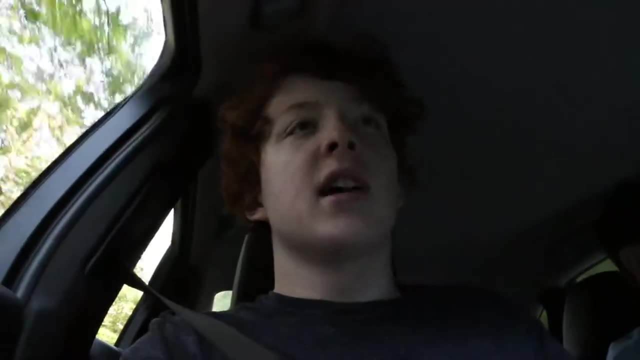 in the meantime, I guess. All right, we are going up this windy road on the way to the top. It's about an hour out of Asheville, which is where we're staying tonight, so we're going to have to go an hour up and an hour down, and hopefully this one is a good experience. 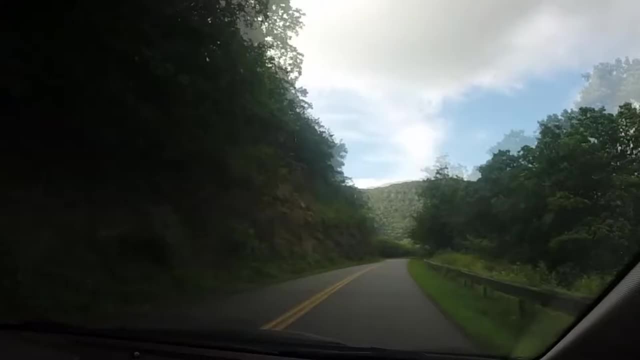 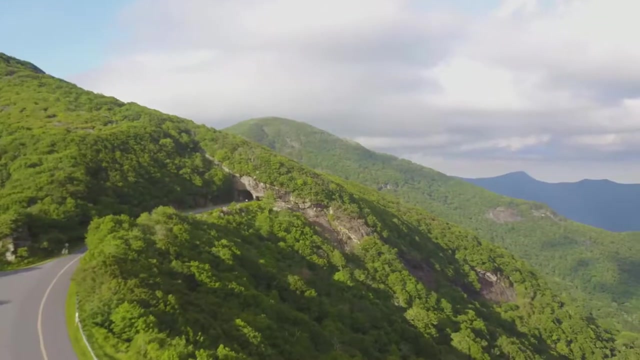 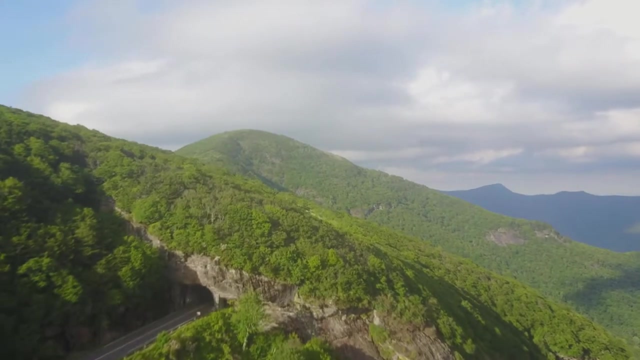 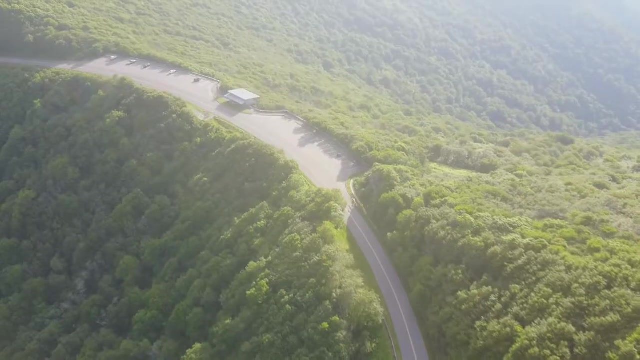 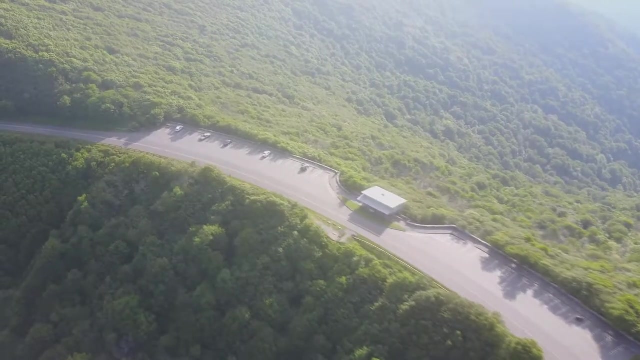 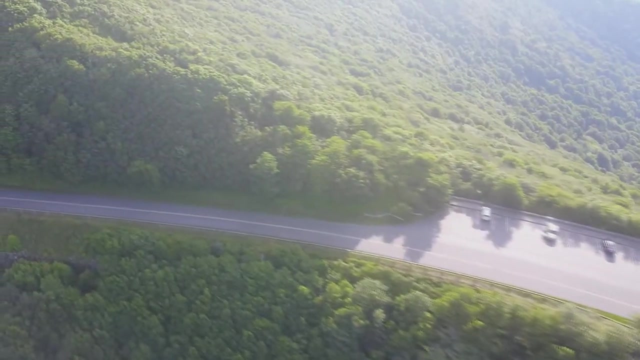 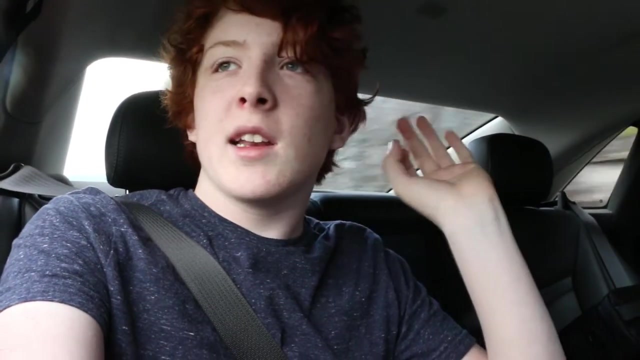 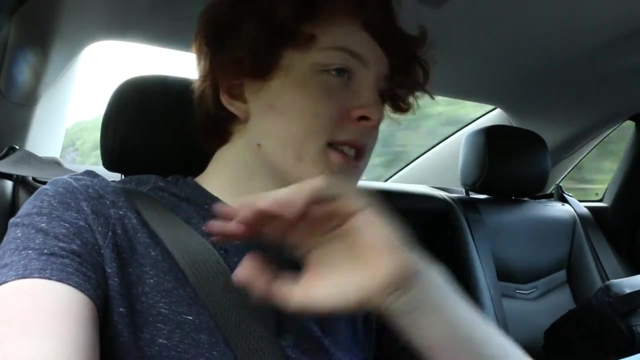 We will see you there. We'll see you guys up there. Okay, so I cheated a little bit with that one. I didn't cheat the government, I didn't cheat the state park, nothing like that. I just I cheated you guys a little bit because 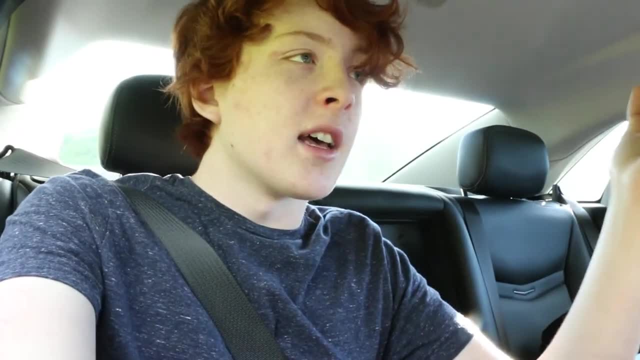 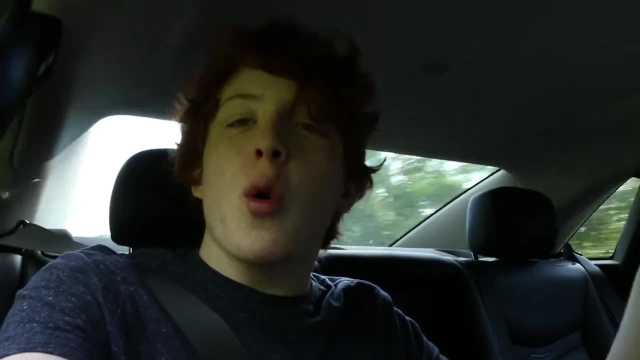 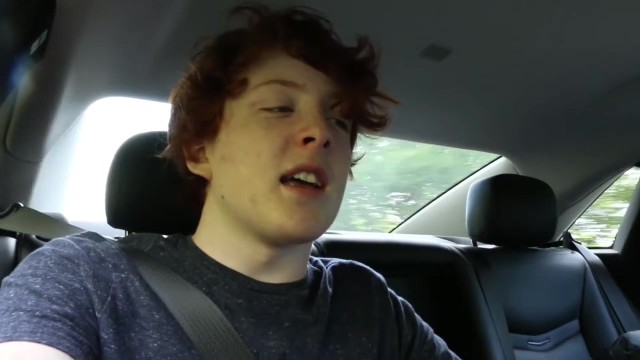 that's actually not the high point in North Carolina. You can't actually even see it in that video. It's just The terrain. it's all quite similar, so let's just pretend that's the high point. This is just the scenery of the drive and let's just pretend. 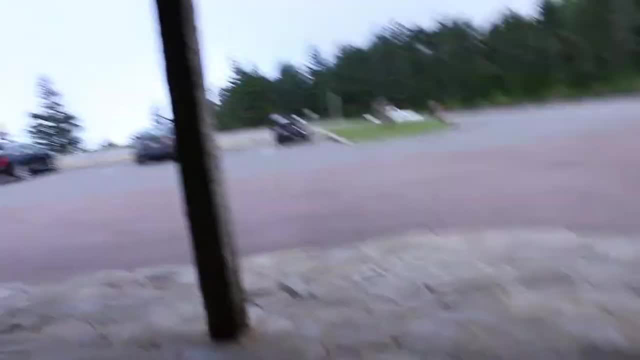 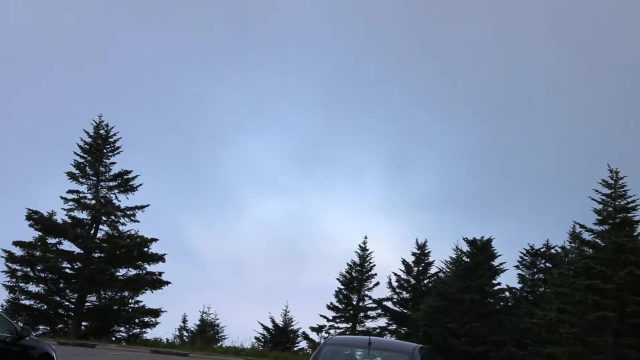 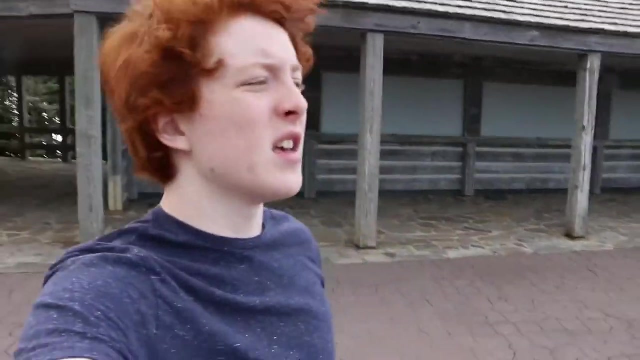 So check this out. There's kind of a ridiculous amount of fog, but it's moving really fast. Can you see that? I mean I can watch it When you're standing here. you can watch it move about 50 feet in 10 seconds. It's crazy. 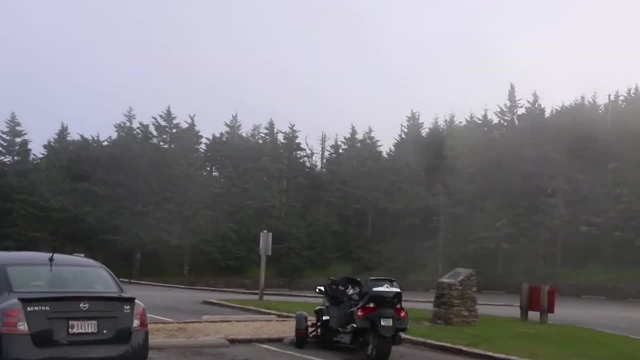 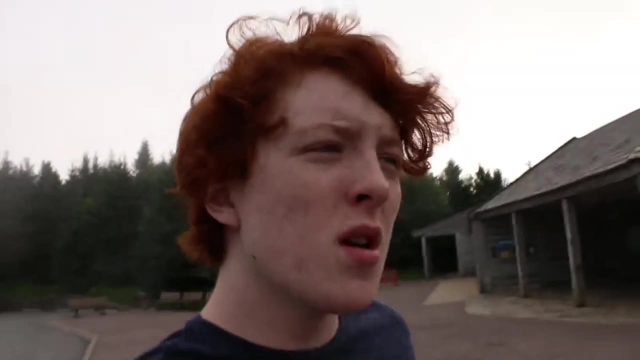 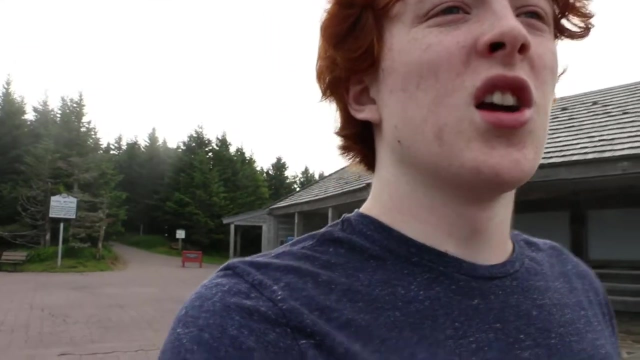 This is the parking lot. Look how fast the fog is moving. You can barely see it, but it's just zooming by As is. there's probably not going to be a view, but the hope is that by the time we get up there- or if not, then then maybe a couple of minutes later- that we're going. 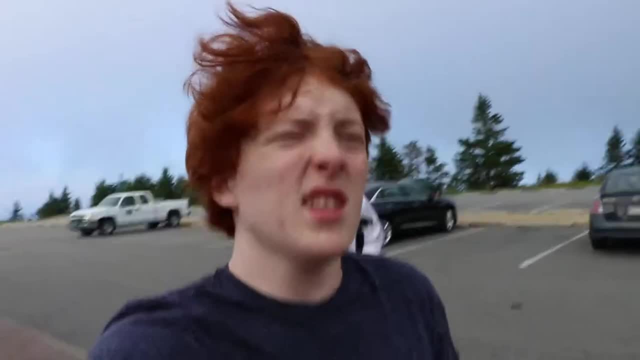 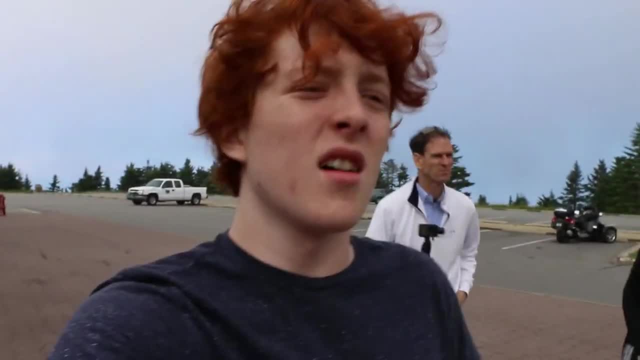 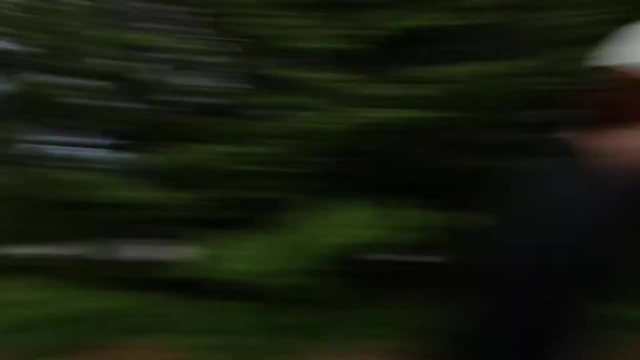 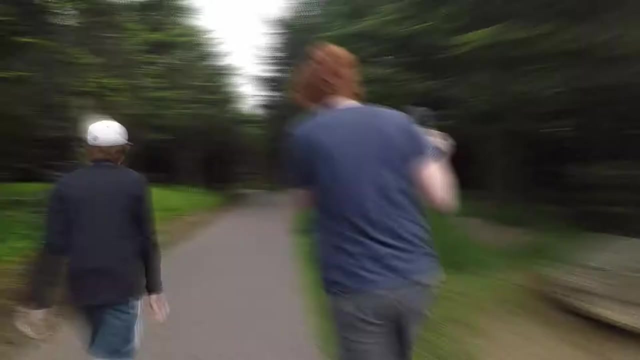 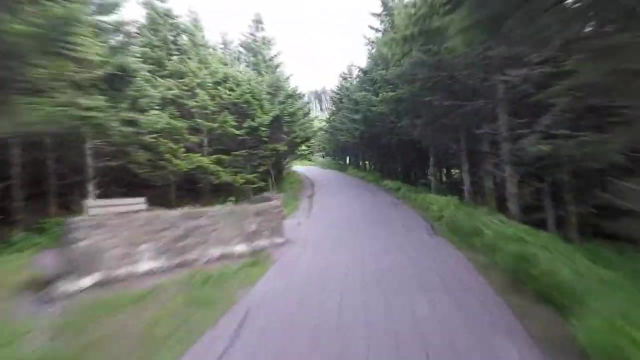 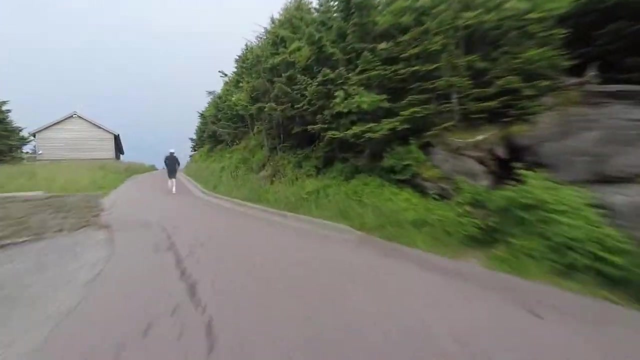 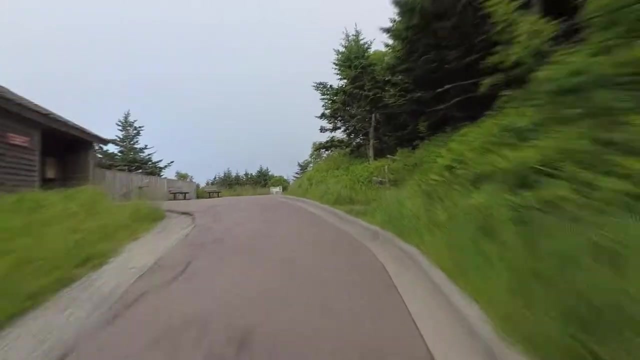 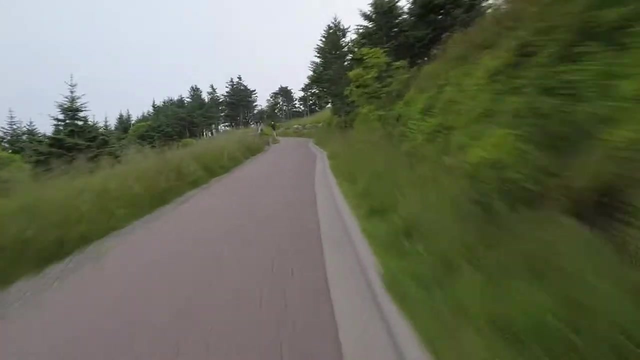 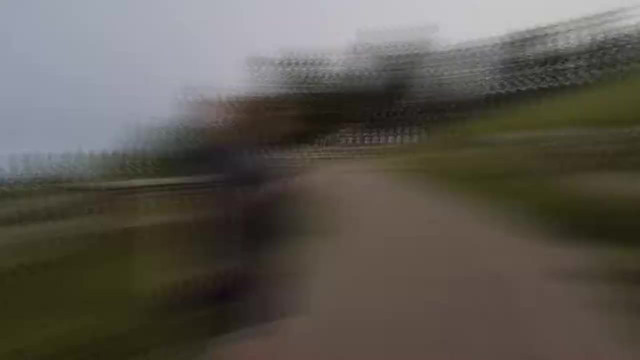 285 yards and judging by that plaque that was over there in the parking lot of the elevation at that exact altitude, it's about 100 feet up. So we're it's all good. Cool, It's cool. Yeah, Thank you. 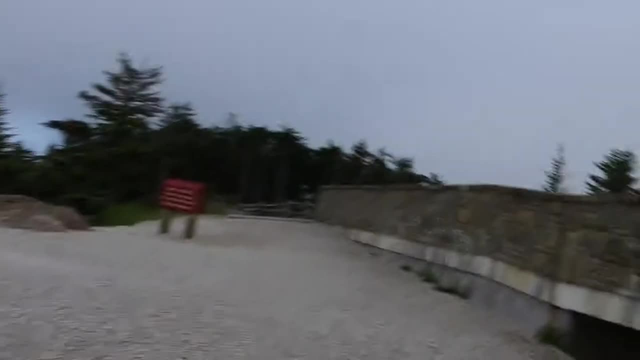 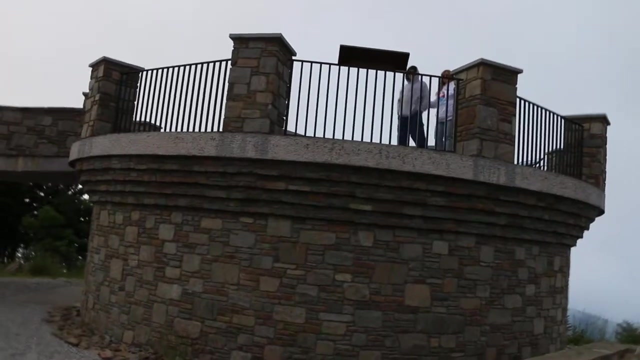 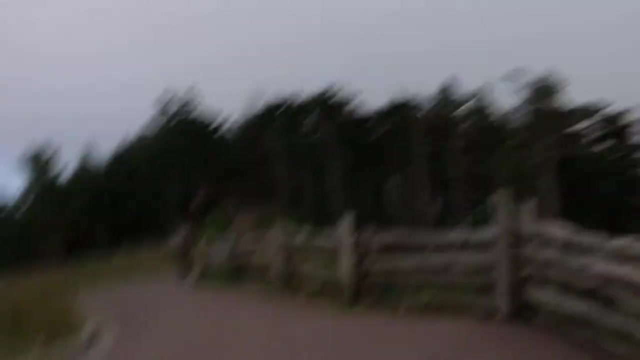 Thank you. Oh, he's buried here because you seem to read it. He was a professor at North Carolina. He died, Sir. Yes, sir, You happen to know where the exact highest point is. Is it under the memorial Memorial? 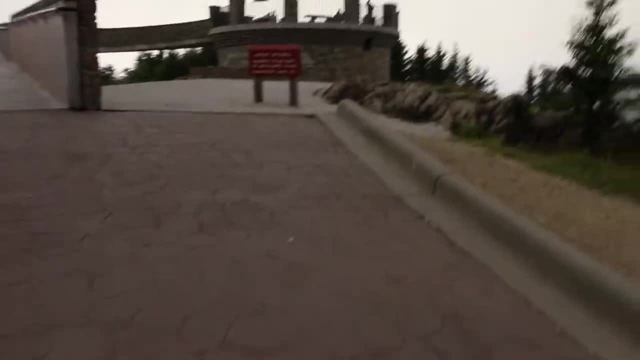 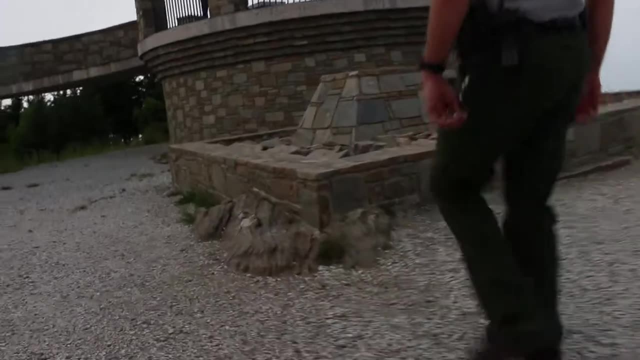 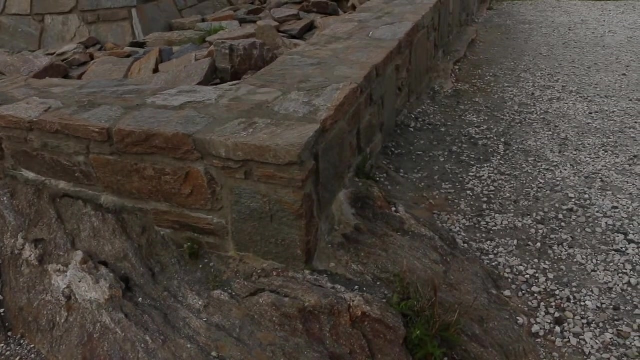 Hard to say with the construction. Yeah, It would be. it would more than likely be on the original rock work where they based this off of: Okay, That's it, Because he's buried, he's supposed to be buried, sort of close. 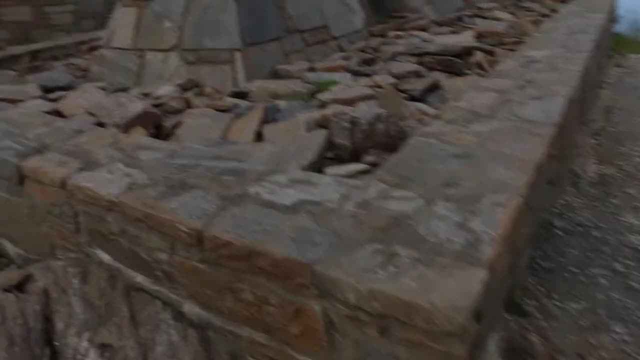 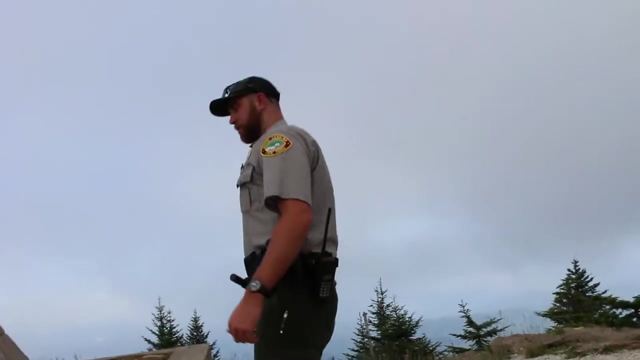 to where he took his measurement from, Okay, But of course over. you know he was buried 160 years ago, so Yeah, He's missing. like these rocks were his original, what they made his original tomb out of.